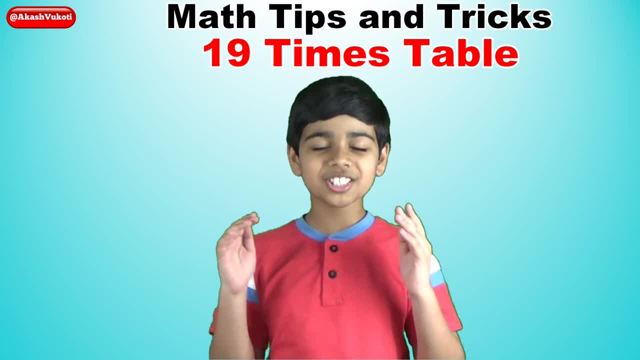 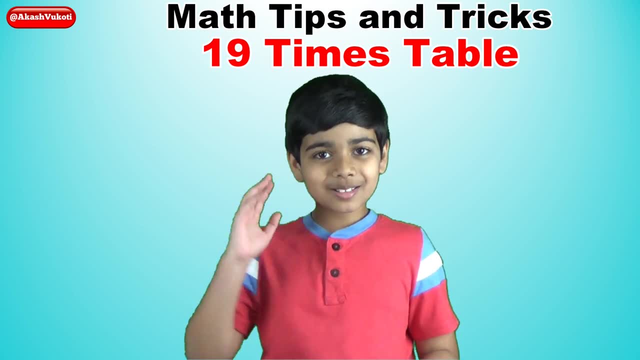 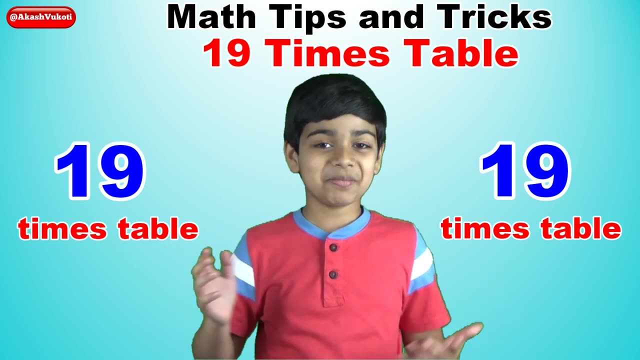 Hello friends, I'm Akash. We have successfully completed all of the multiplication tables from two to nine. So today, in the math tips and tricks series, we are going to be learning the trick for the 19 times table. Yep, the 19 times table. There's actually a really neat trick for. 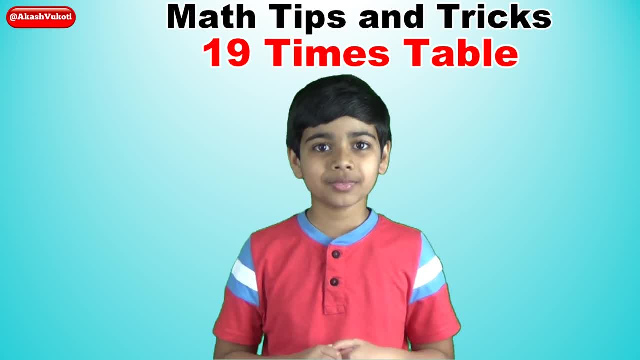 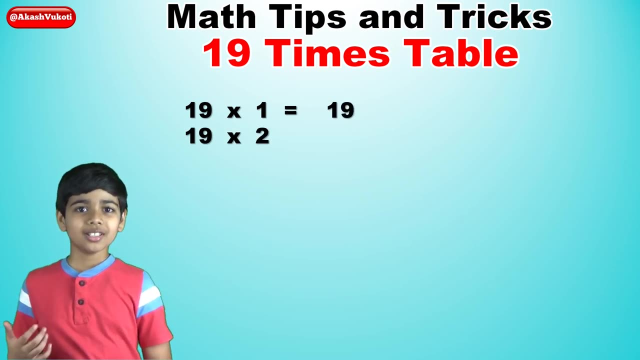 learning this one. so today we'll be going over it. But before looking at the trick, let's recite the 19 times table from, of course, the very beginning. 19 times 1 is 19.. 19 times 2 is 38.. 19 times 3 is 57.. 19 times 4 is 76.. 19 times 5 is 95.. 19 times 6 is 114.. 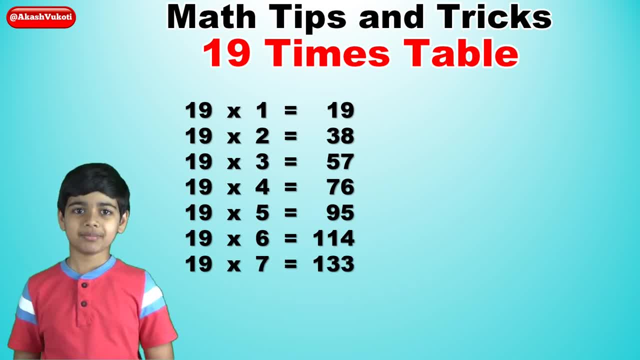 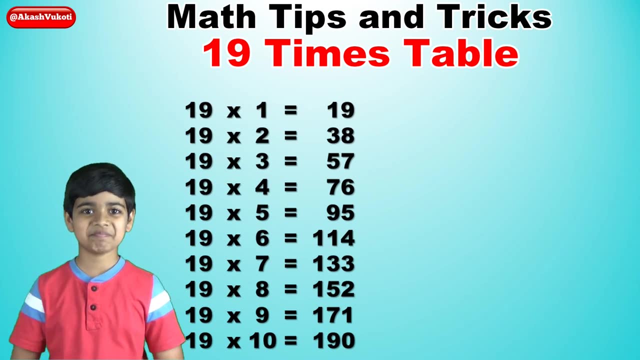 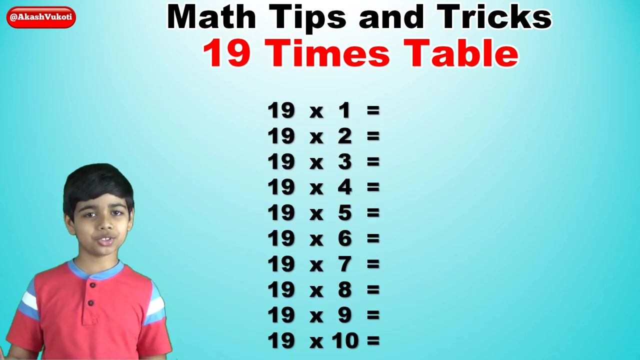 19 times 7 is 133.. 19 times 8 is 152.. 19 times 9 is 171. And finally, 19 times 10 is 190.. Now we can start. Let's start by writing 19 times 1,, 19 times 2, and so on and so forth. 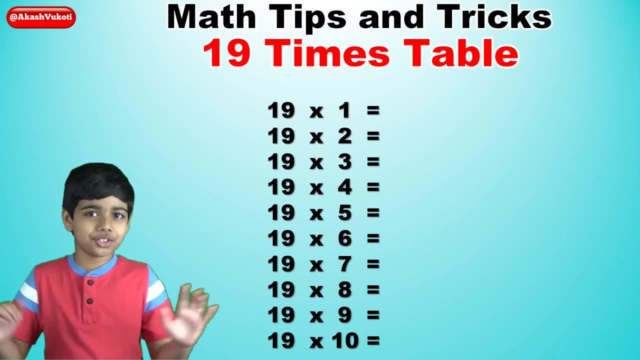 as written here in a column like this. You don't actually have to do it, I'm just writing it here for the sake of actual you know. So next for the ones digits. This is the trick. We just write all of the numbers from 9 to zero. 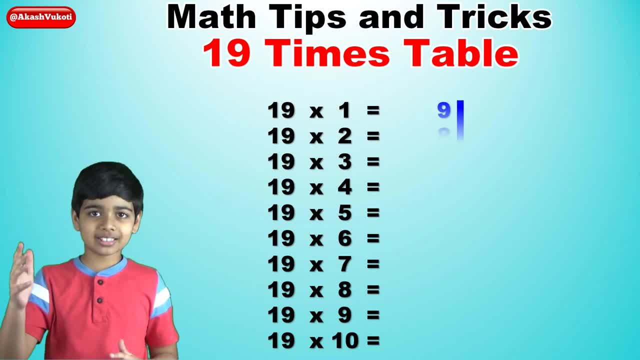 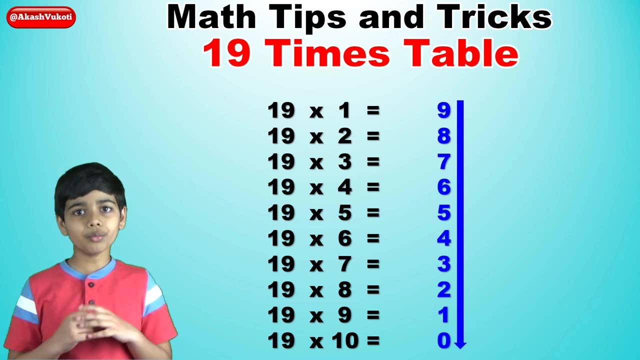 which is descending order. So nine, eight, seven, six, five, four, three, two and zero. Now for the tens digits. all we have to do is just write the odd numbers from 1 through 19. I mean odd numbers from 1 to 19 in ascending. 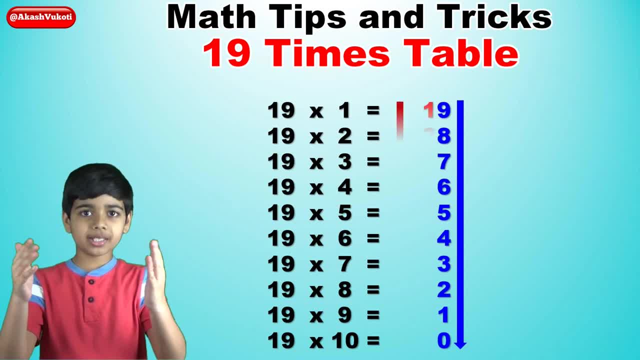 order, of course. so that means 1, 3, 5, 7, 9, 11, 13, 15, 17 and 19, and now, if you take a look, you have surprise, surprise, the 19 times table. take a look. this is a really simple and easy way to learn the nine times, the 19 times table. take a look.